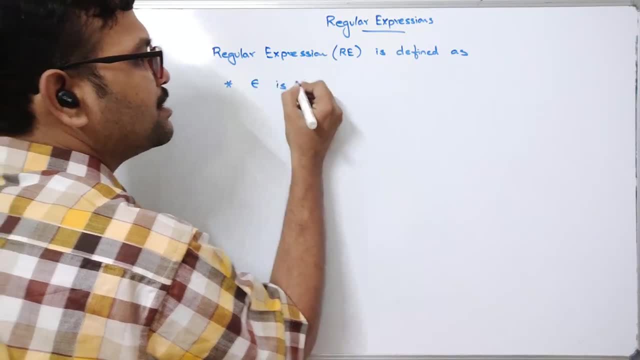 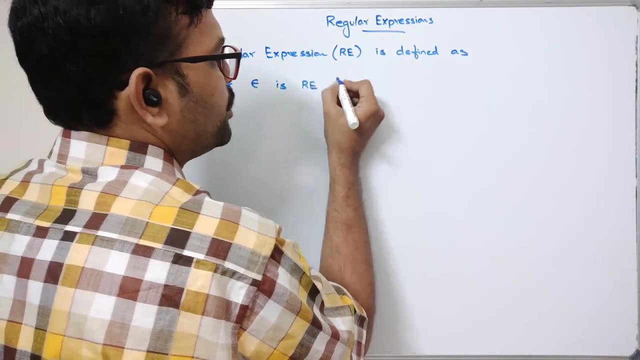 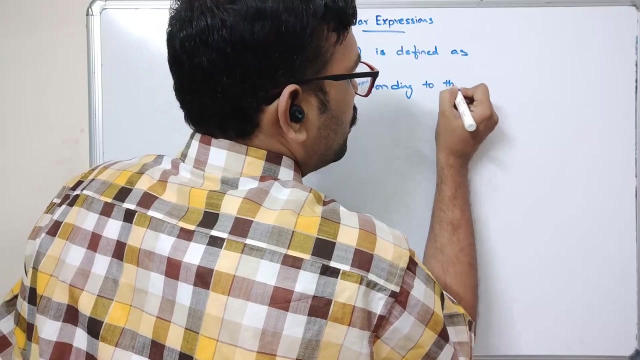 So epsilon is a regular expression. we know the epsilon. epsilon means the empty string. So regular expression corresponding to the language, to the language L is equal to empty string. Team C In a low bit set of variables or in the basic sense, the only variable that will be an empty string. 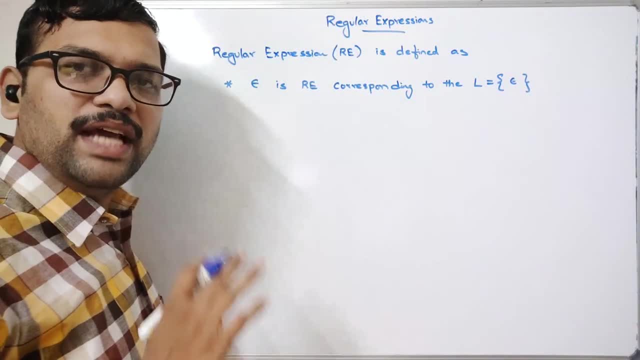 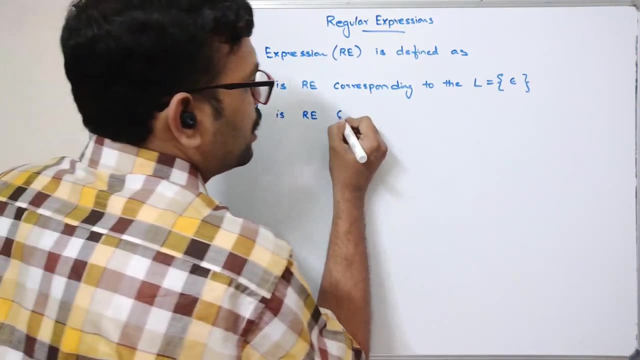 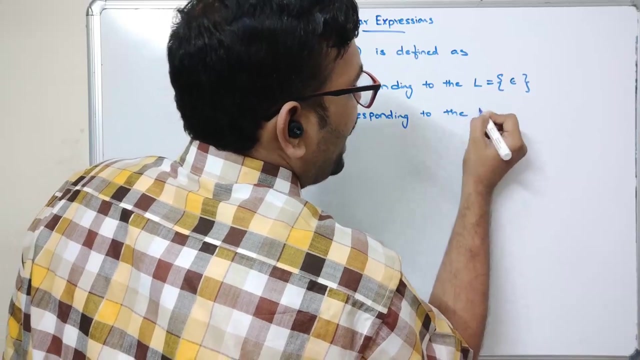 So regular expression is a regular expression步 pela string corresponding to the language l is equal to empty string. and one more point, that is a phi is a regular expression corresponding to the language with the empty set: empty set. so you just observe, both are different. first one is: 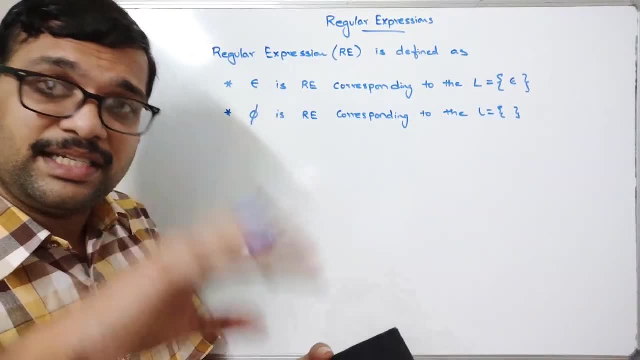 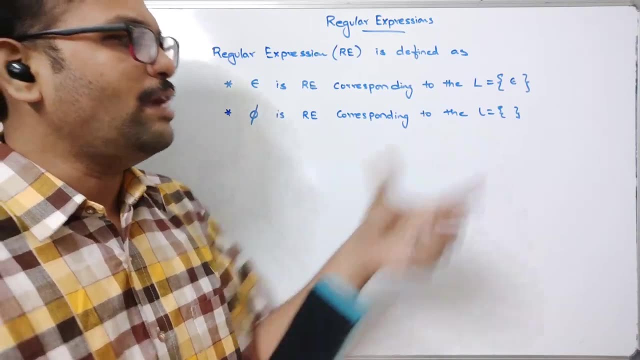 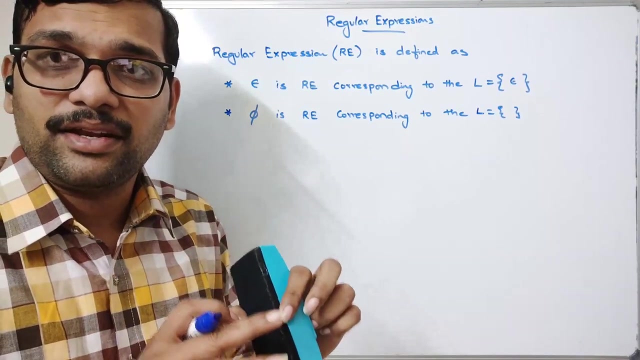 an epsilon. that means null string. that means there is a string but the length of the string is zero. but here, coming to the phi, it is called a regular expression corresponding to the language. l is equal to empty set. that means there is no string. empty set: okay. empty set. that means language is. 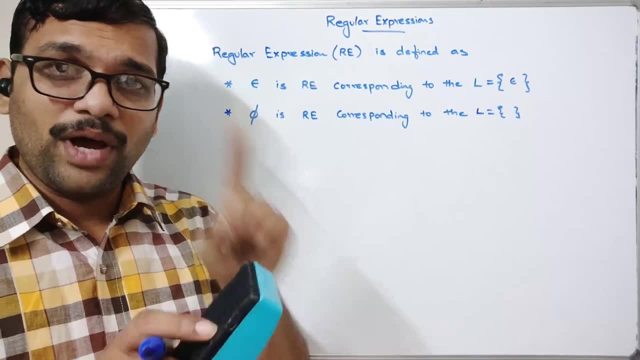 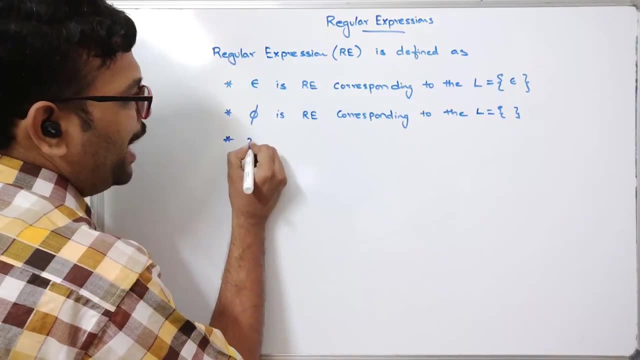 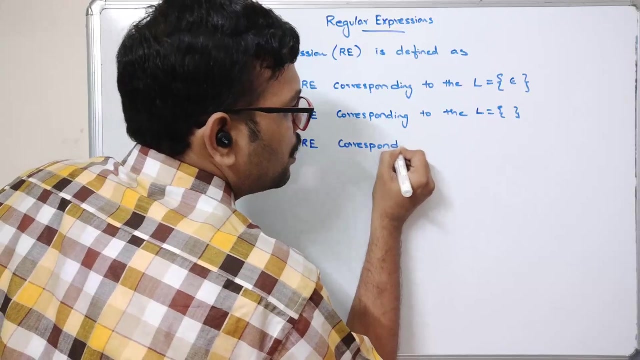 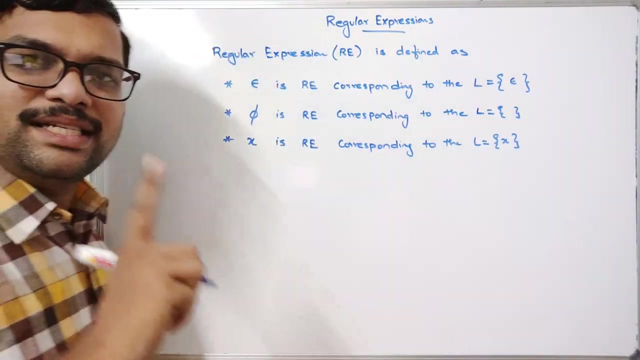 not having any string. but here language is having a only one string where the string length is zero. that means a null string, epsilon and the next one, so x, is a regular expression corresponding to the language having only one string called x, only one string called x, only one string, right. and so if 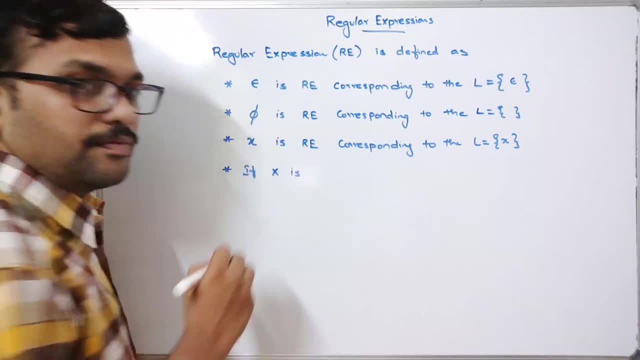 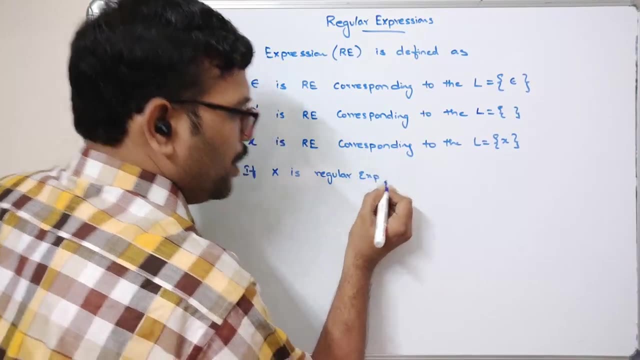 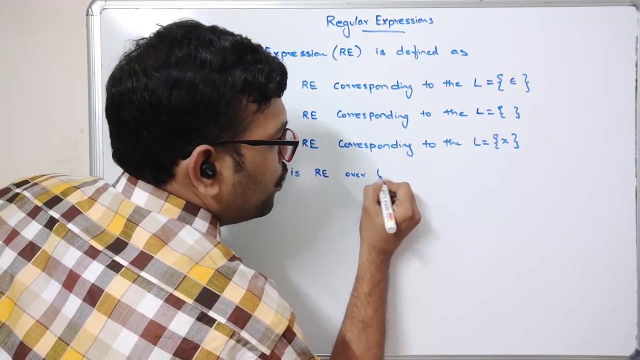 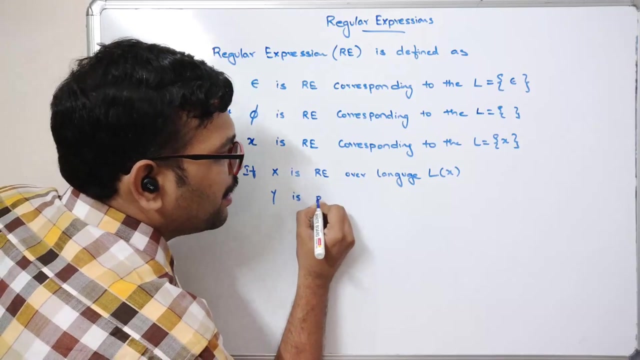 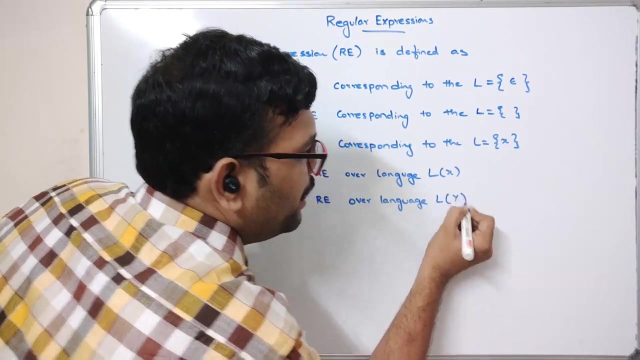 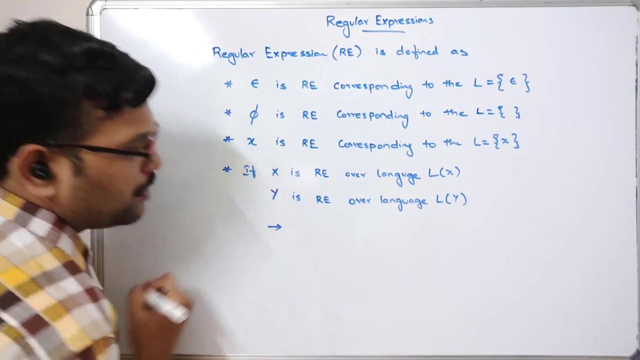 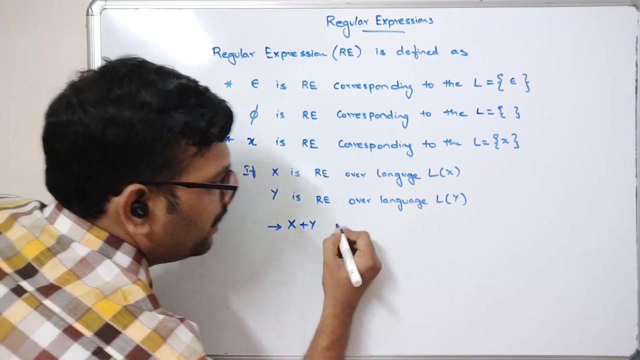 x is. if x is regular expression. sorry, i will write this over a language l of x, and y is a regular expression over language l of y, then, then, so this is most important. the first one: x plus y. x plus y is a regular expression over language l of x, and y is a regular expression over language l of y. 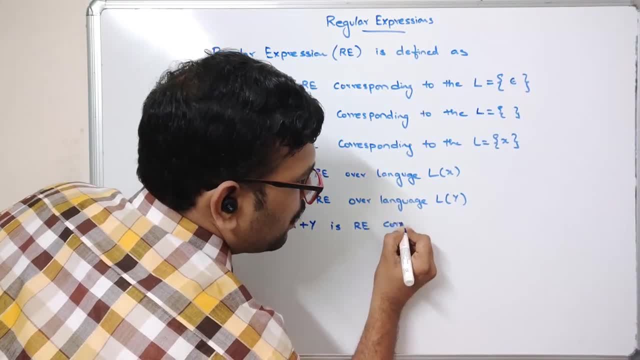 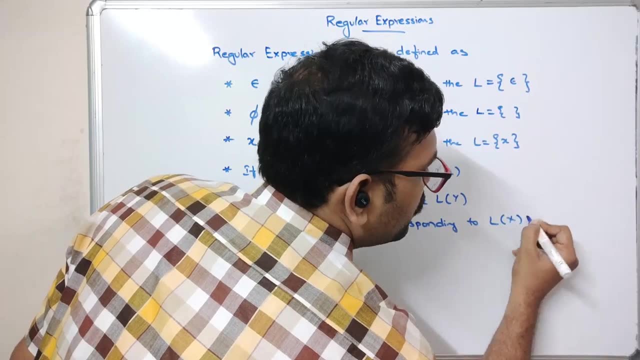 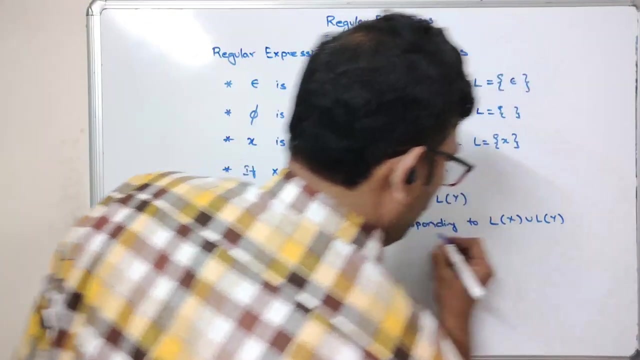 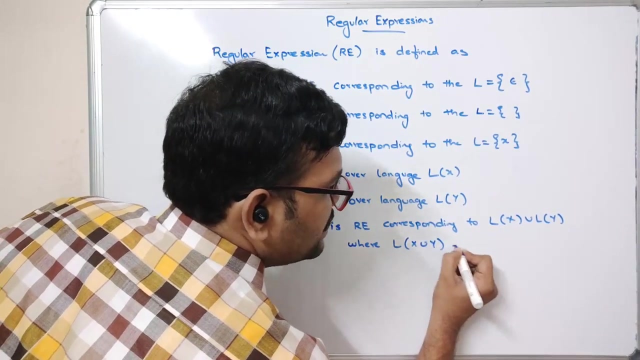 is the regular expression corresponding to l of language nie Cross union language y. l x union once y, which is the regular expression corresponding Toby x union language. why language of X Union language? why, where language x union language, why is equal to the language language of x union language of y. 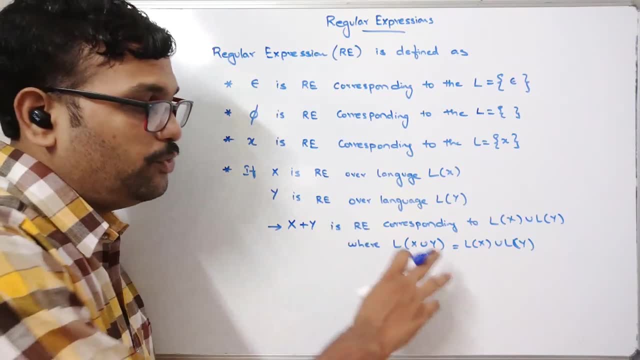 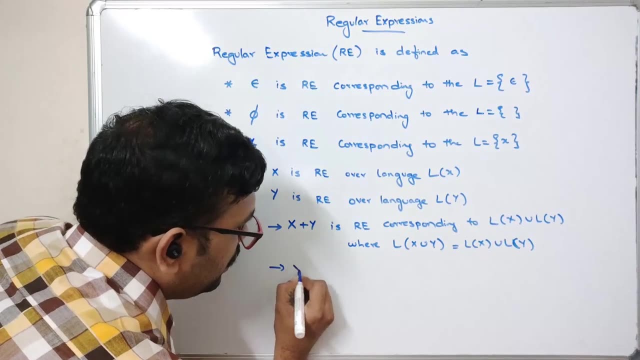 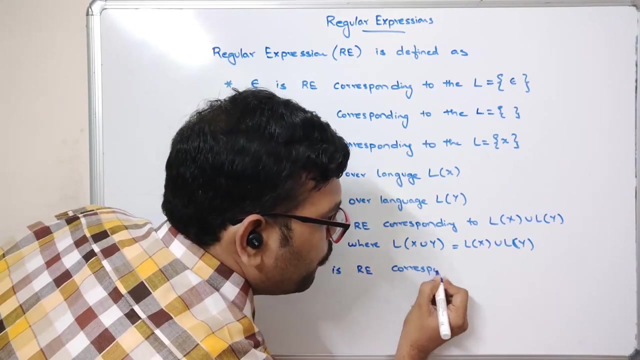 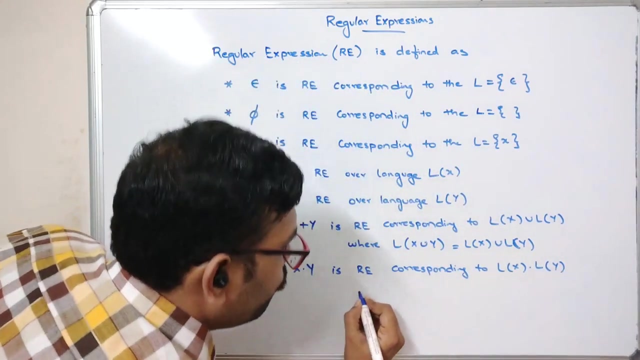 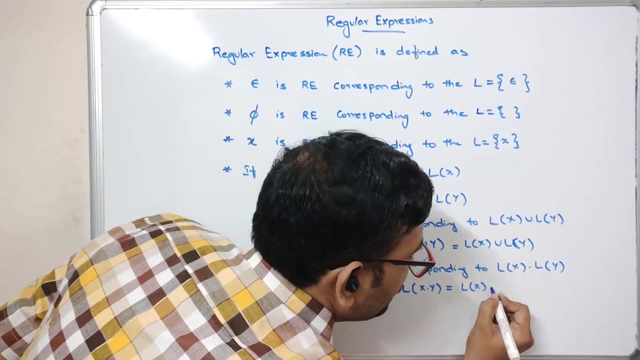 well, So this is a union. okay, this is a union. So if it is a union, we will represent it as a plus x, plus y. And the next one, xy, is a regular expression corresponding to L of x into L of y, where L of xy is equal to L of x into L of y. right, 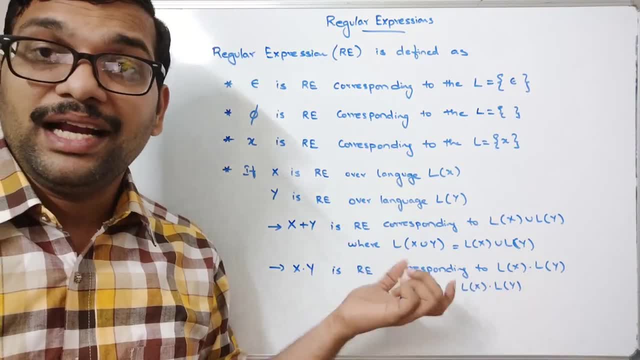 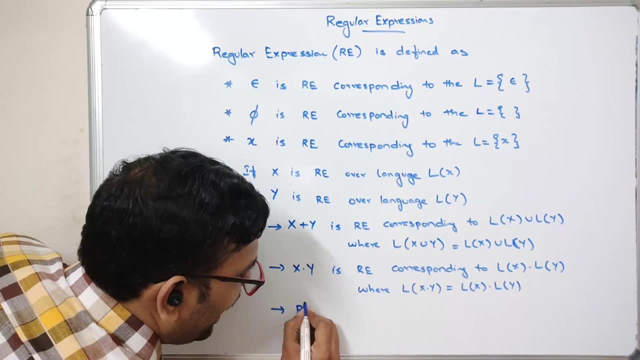 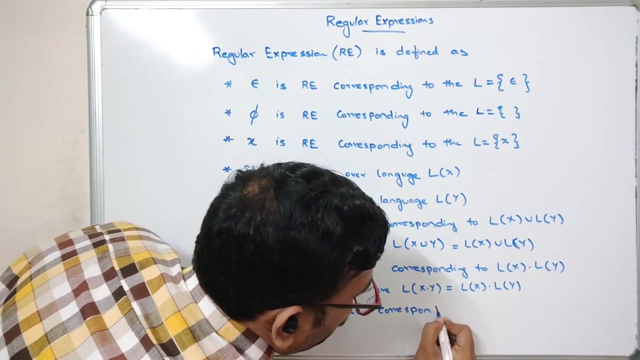 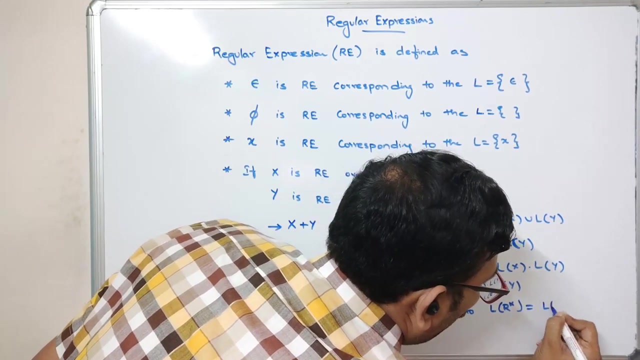 So this is nothing but a product, which can also be known. It can also be known as a concatenation. So this is a union and a concatenation, And the next one is a closure, closure. So R star is a regular expression corresponding to language. L of R star is equal to L of R whole star. 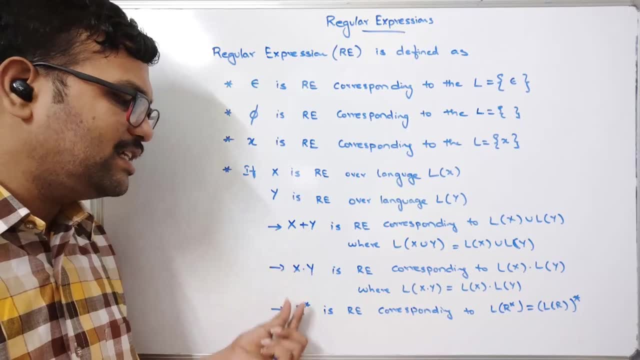 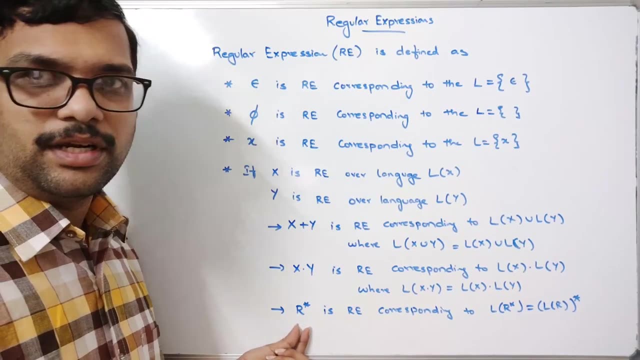 So this is a closure. This is called a closure, Union, concatenation and a closure If it is a union. If it is a union, we will represent with a plus. If it is a concatenation, we will represent with a product and closure right. 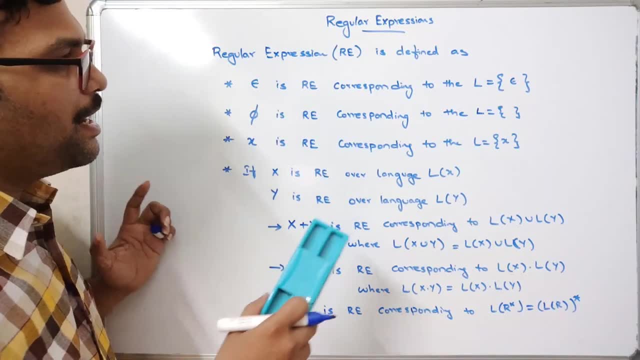 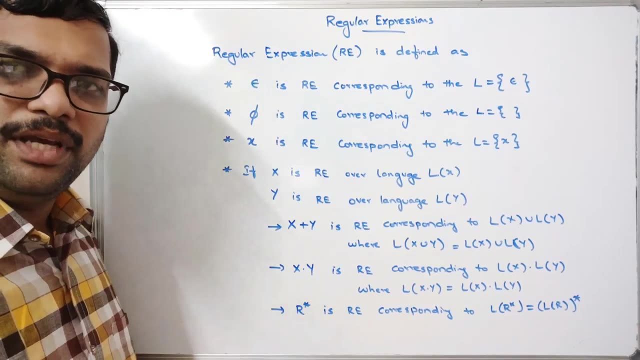 Star represents the closure, So this is a regular expression, right? So I hope you are having any doubt about this regular expression. I will give you an example so that everything will be clear right Now. the second thing is: what are the applications? 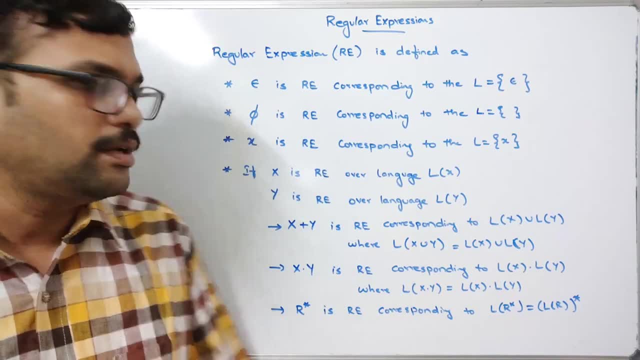 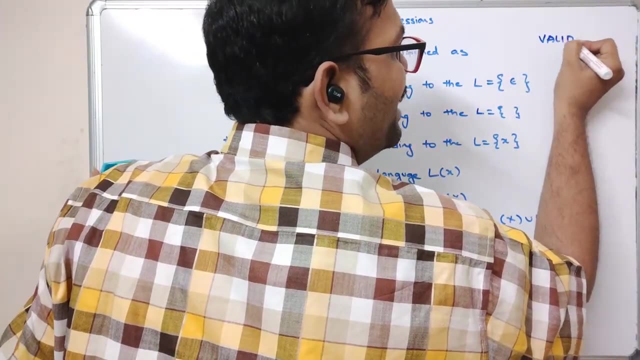 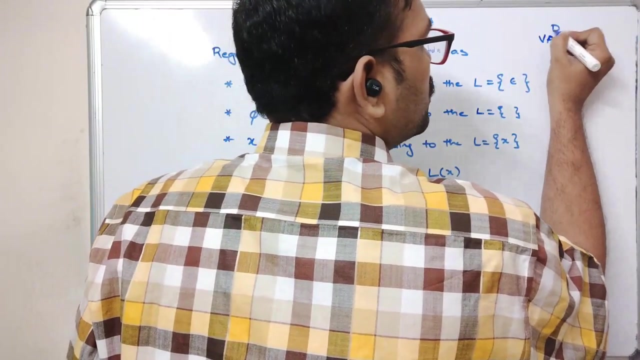 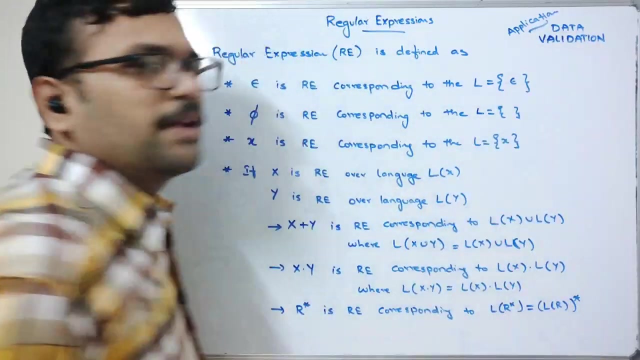 That means where we are going to this, going to use this regular expression. So one application of this regular expression is validation, data validation. So in this data validation, we are going to use the regular expression, Best example. so this is the application: data validation. so this is the application for regular expression. application for regular expression. 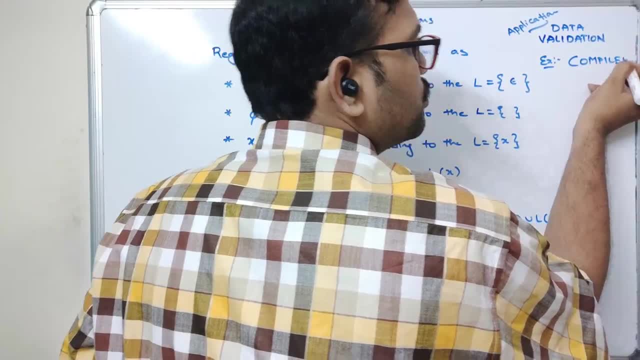 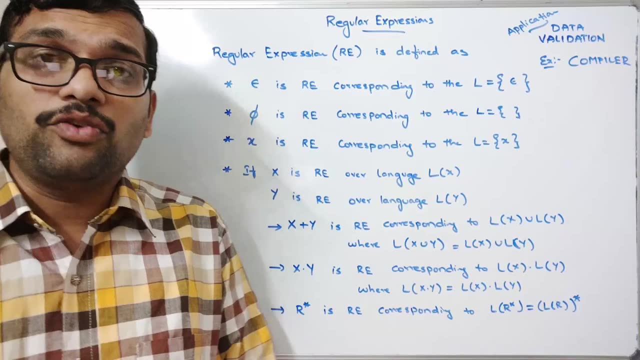 So example: compiler. So we have now gone about the compiler. So the compiler will be used to convert from one language to another language executing any C programming. So first we are writing the program and then we are compiling the program so that the object root will be generated without any. 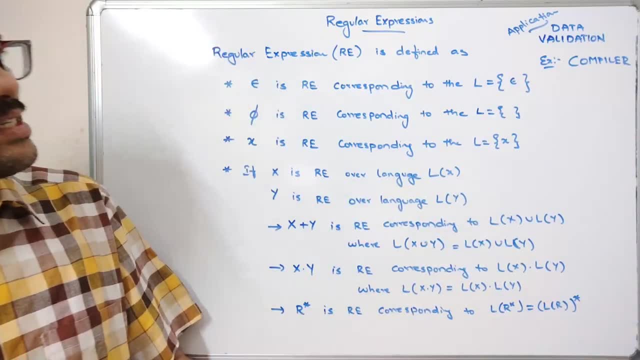 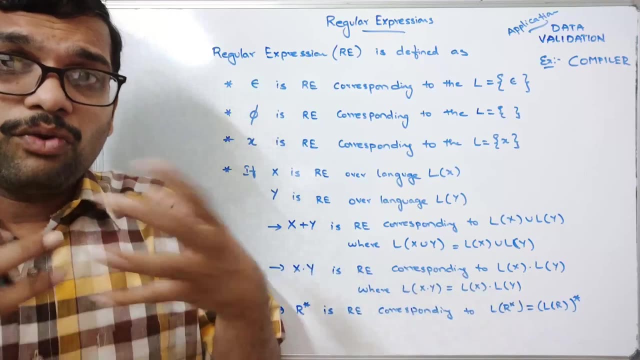 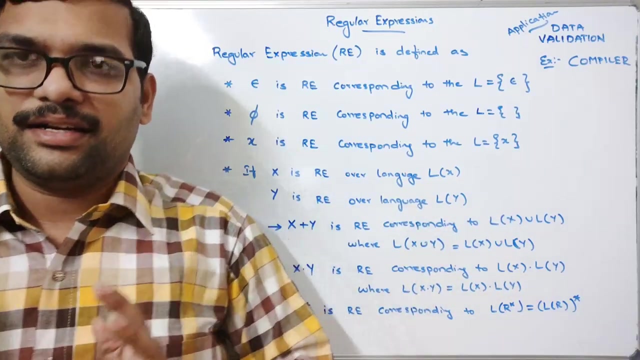 syntax errors and then we are executing the program. So in this concept, compiler's concept, the compiler will set some sort of rules right And we need to write the program that obeys that particular rules. If any rule is violated, automatically we will get the syntax error, So that data validation 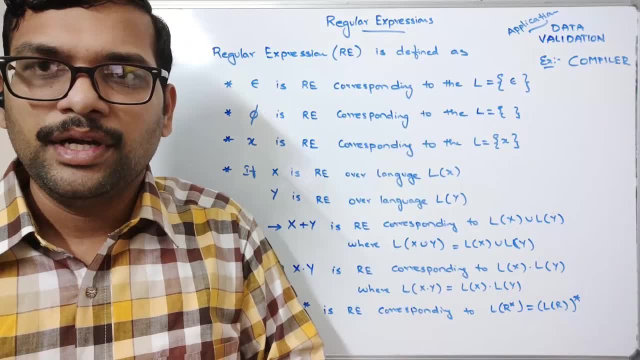 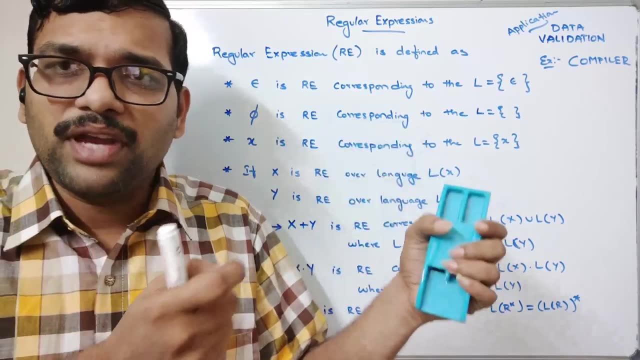 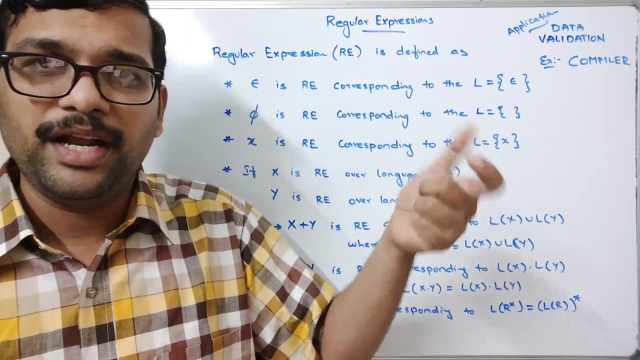 will be done with the help of this regular expression. So if you write the program- complete program- first, the program will be divided into small tokens and each token will be compared with the compiler set, I mean the rules set by the compiler. So this comparison will be done with the help of regular expression. And if 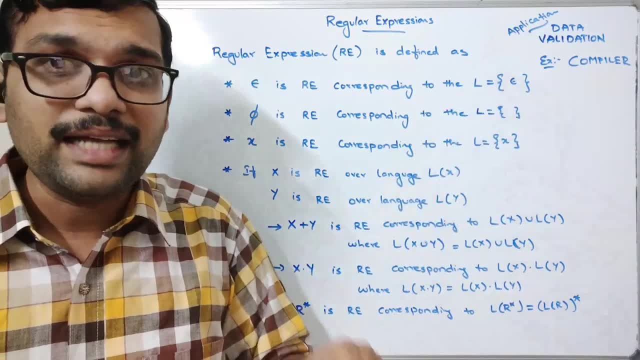 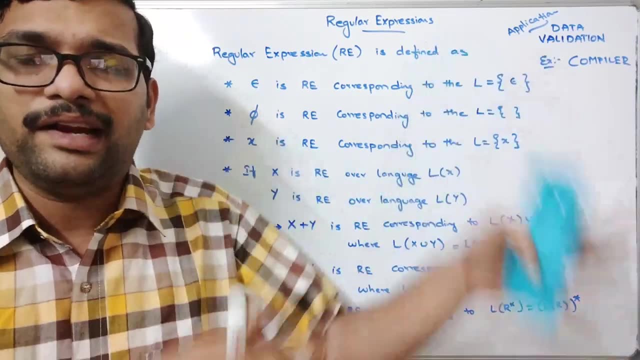 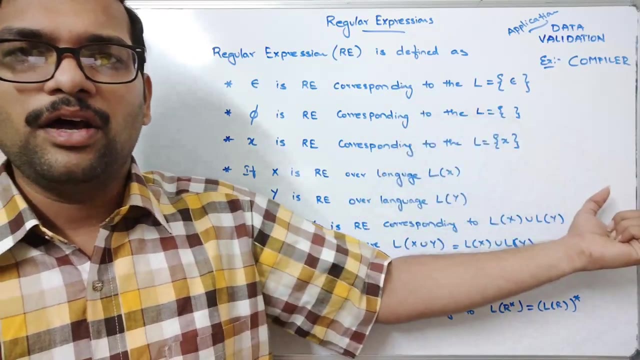 any rule is violated, automatically we will get the syntax errors. So you know about the syntax error. We will get the syntax error only if we violate the rule while writing the program. It doesn't check any logical errors, Just it will compare the programming instructions with the rules set. 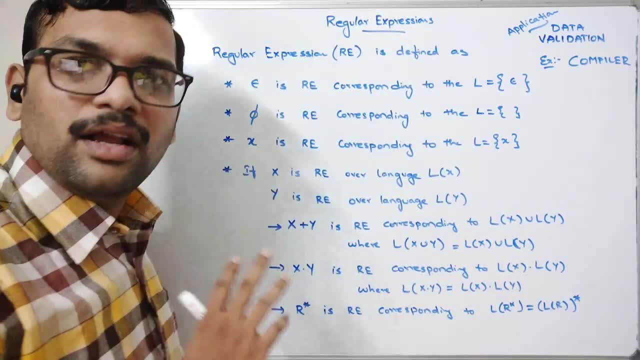 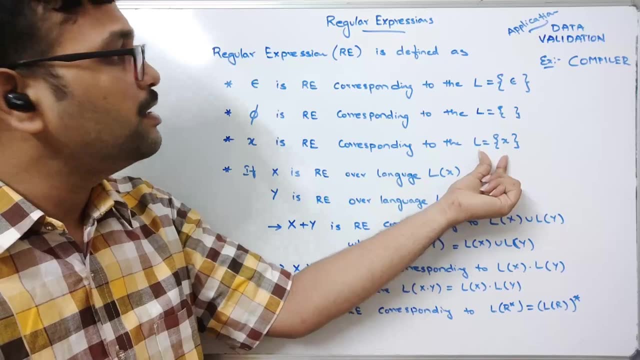 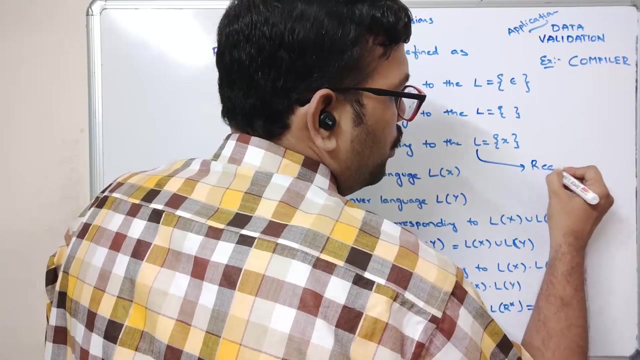 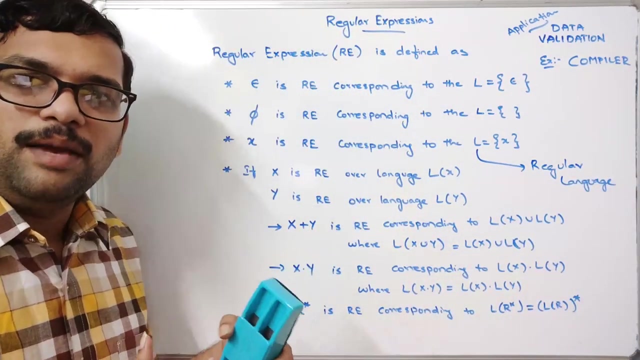 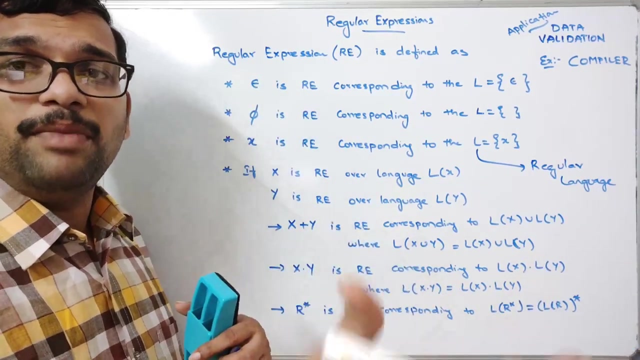 by the compiler right. So that is the best example for this regular expression. And whatever the language, whatever the language we are writing for this regular expression is called regular language. So this L is called regular language. So previously we are discussing about the finite automata and we are writing some sort of language and in that language we are writing some strings which are accepted by that particular. 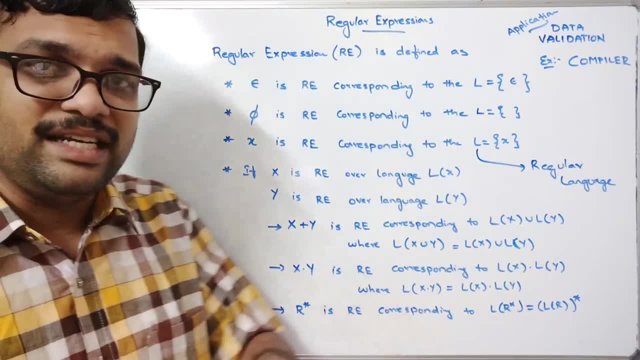 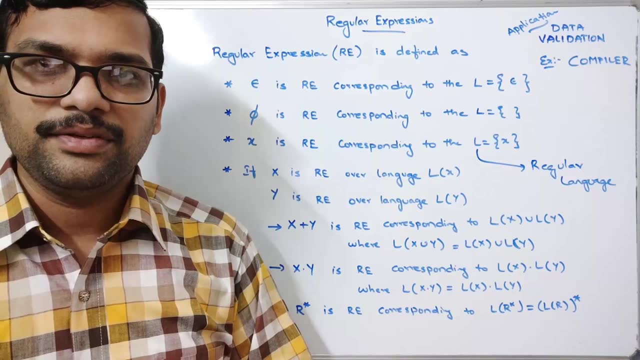 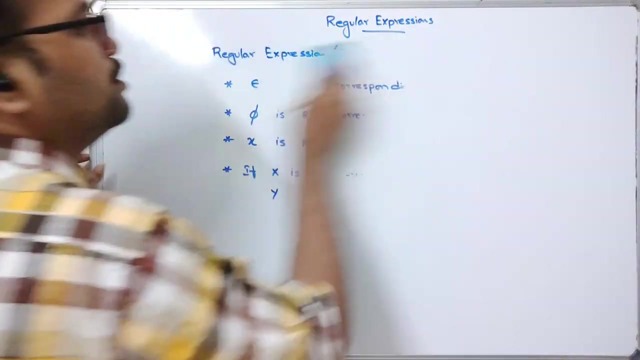 finite automata. that is called a normal language. And if the strings of a language satisfies these regular expressions, that language we call it as a regular language right Now. now see what is a regular language. So hope you understood about the definition and 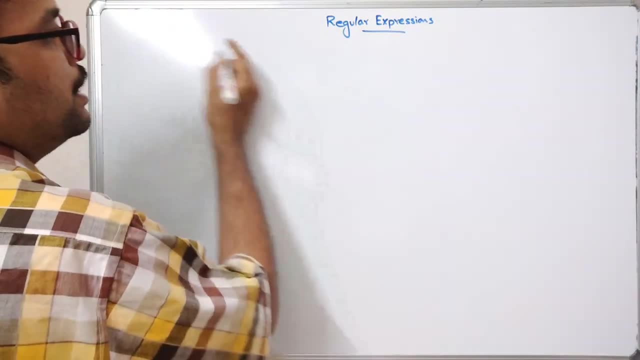 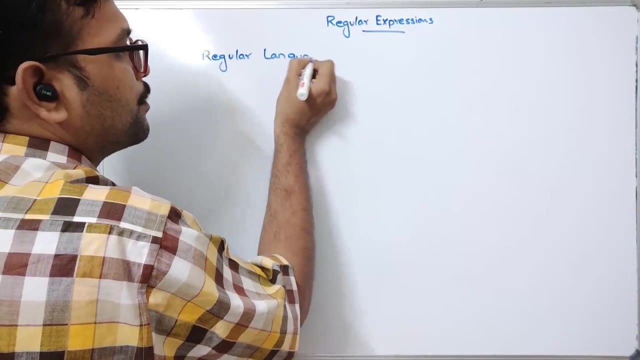 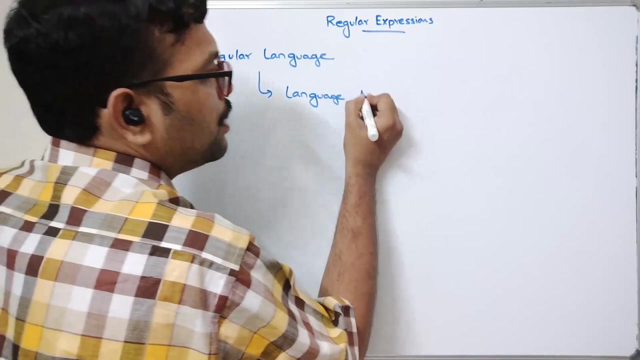 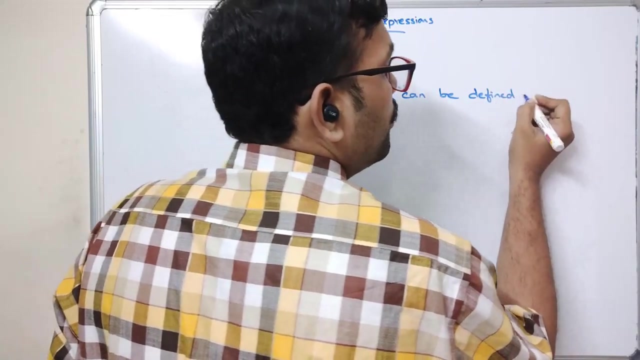 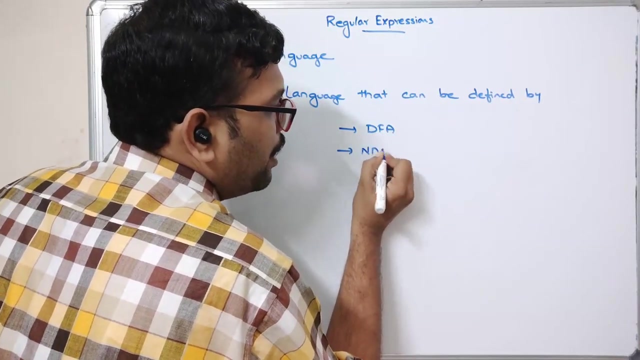 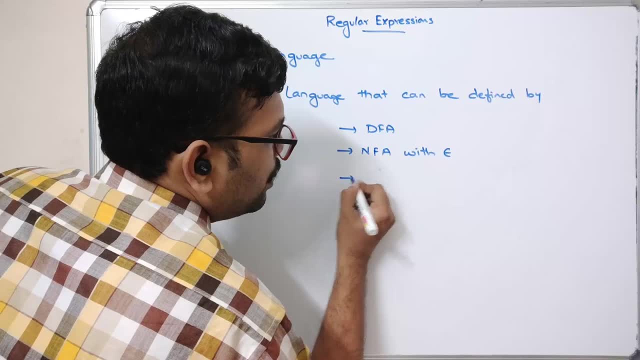 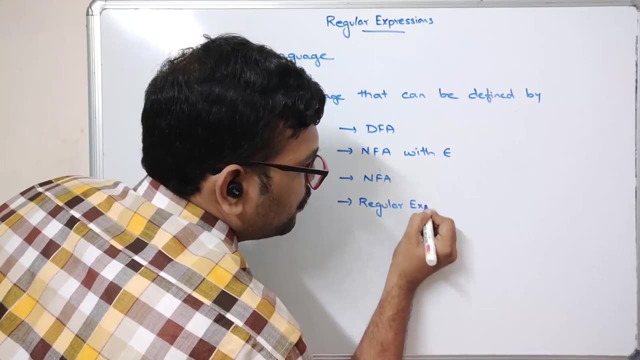 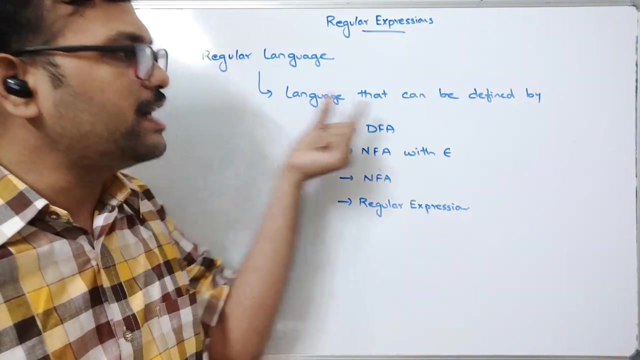 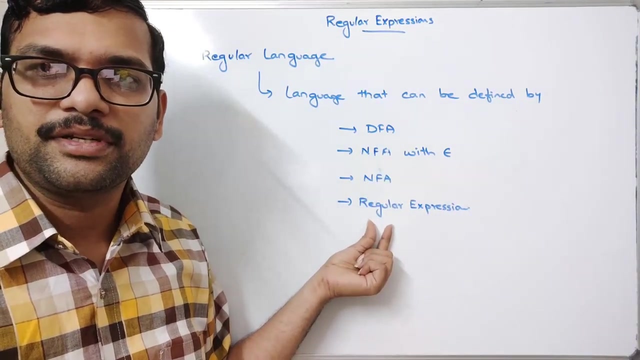 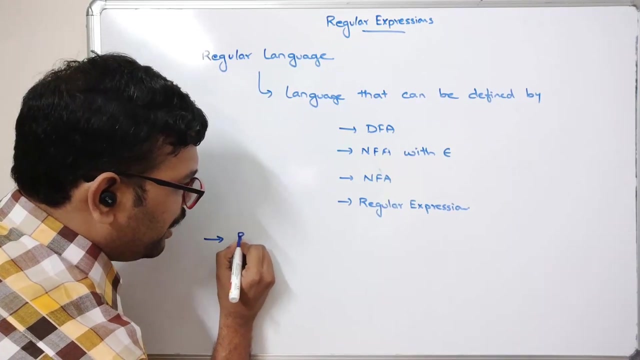 NFA or the regular expression or the regular expression. So the regular language is a language that can be defined by either DFA or NFA, with epsilon or NFA or the regular expressions. Now we will see the example. so we need to write the regular expression denoting language. 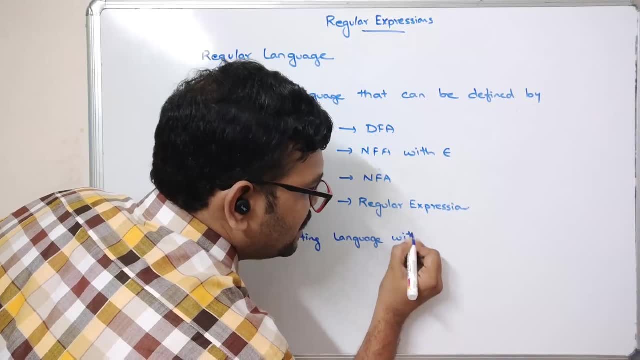 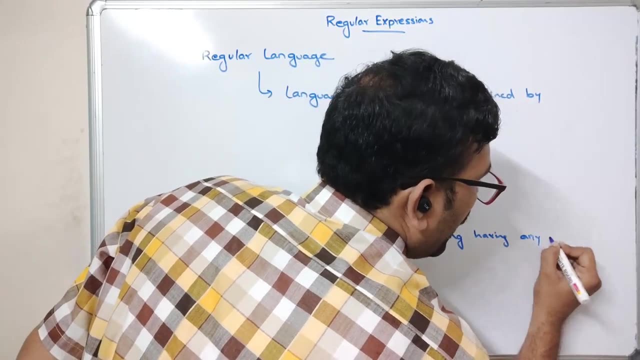 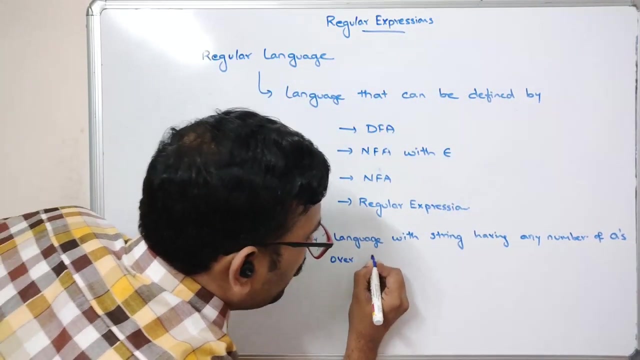 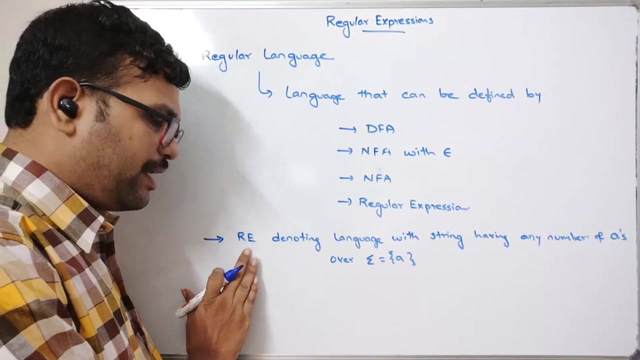 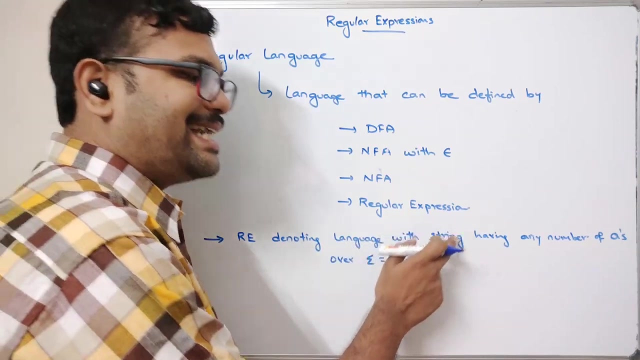 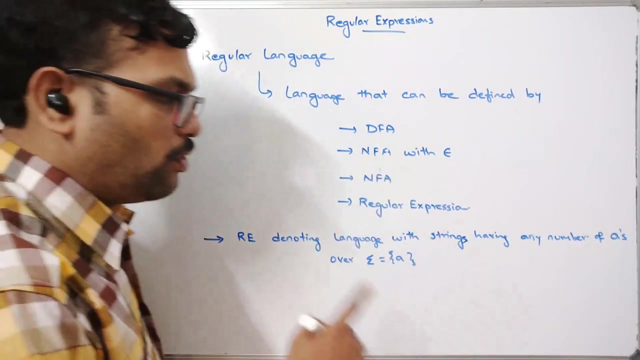 with a strings having any number of A's over alphabet A, See here, in this example, we have to write the regular expression. see RE means regular expression. right, we need to write the regular expression which denotes the language With strings, with all the strings having any number of A's. so if you want to write, 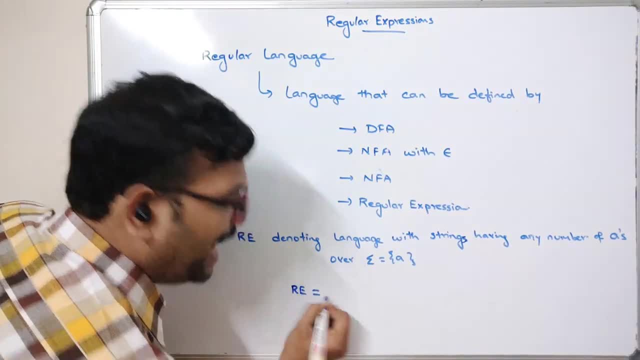 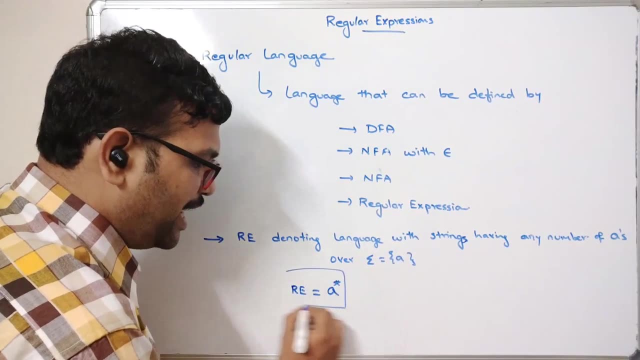 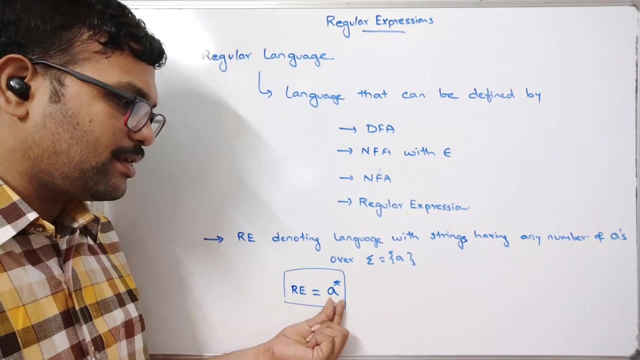 the regular expression for this one, the RE will be any number of A's. that means 0 or more. so simply we can represent it as A star. so A star is the regular expression. so this is in the form of algebraic right. so A star is the regular expression which accepts all. 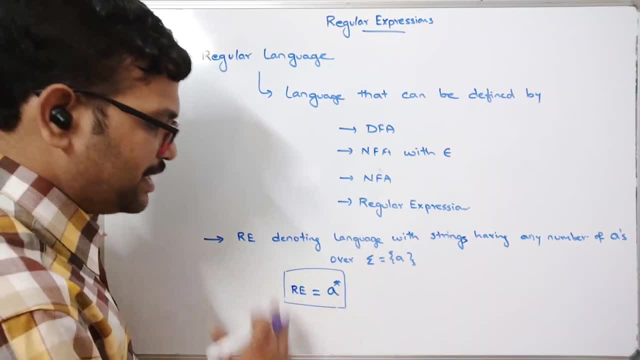 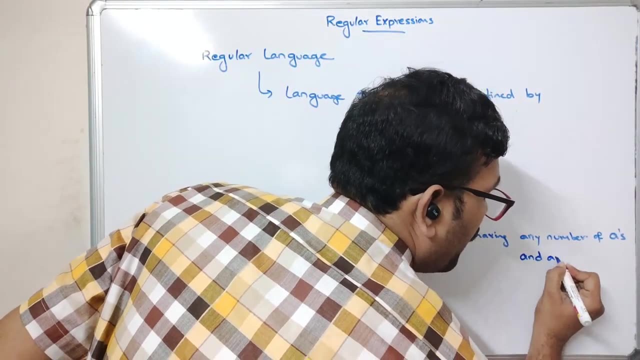 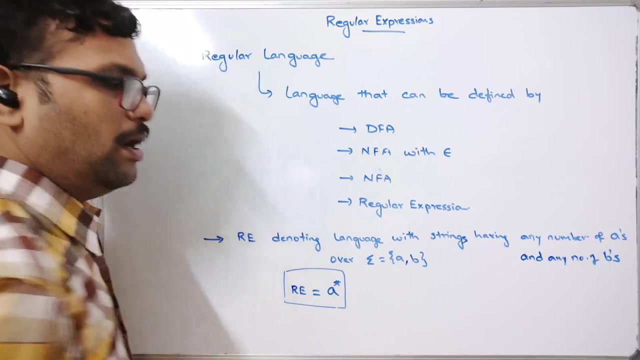 the strings having any number of A's. see the same thing, same example. I will just extend it one: any number of A's and any number of B's over the input symbol A and B. now, what happens here? any number of A's and any number of B's, so anything can be happened. 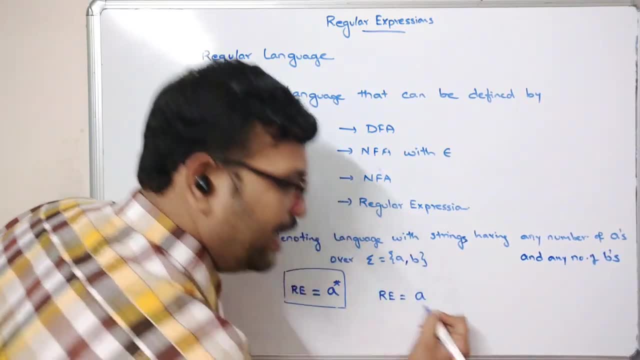 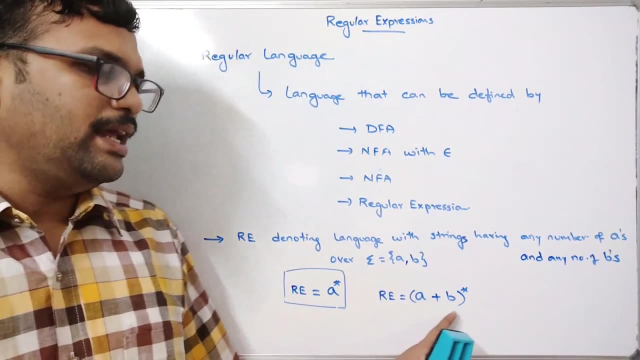 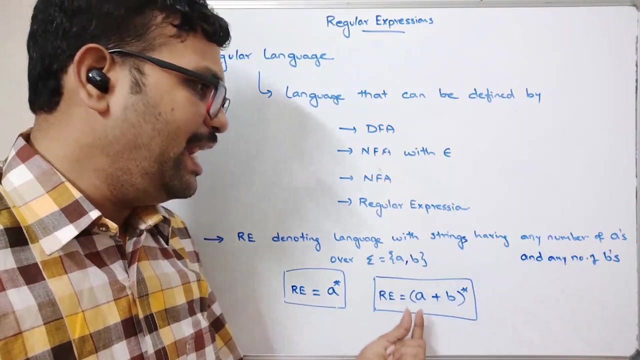 right now the regular expression will be any number of A's or any number of B's over the input symbol. A that means star, so any number of A's and any number of B's. so this is one regular expression which accepts all the strings having any number of A's and any 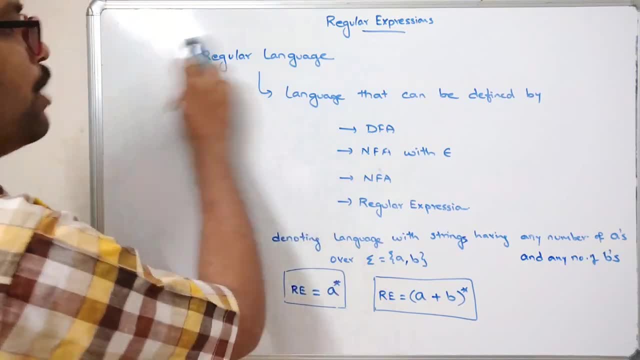 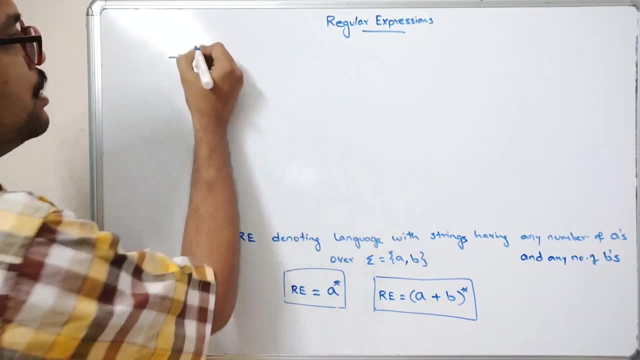 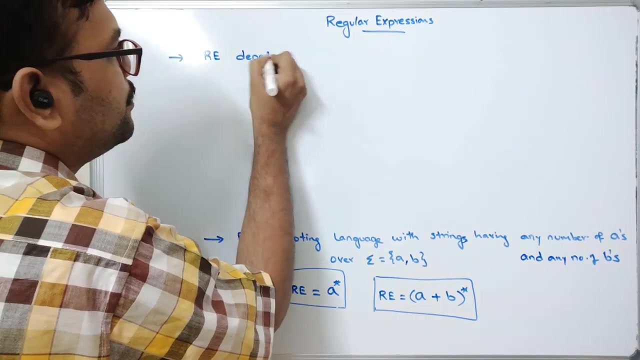 number of B's right now. one more example, and just I will close, and in the next session we will see a few more examples. Now the next one. so we need to write the RE. we need to write the RE so denoting: 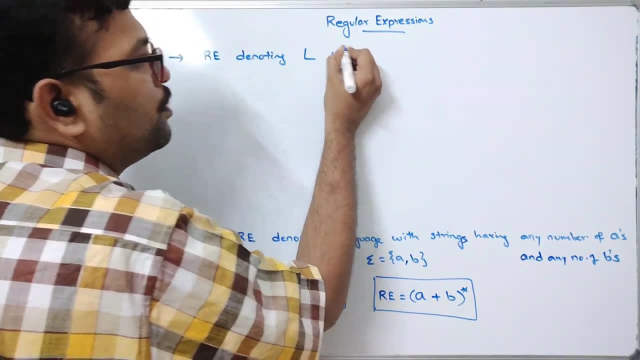 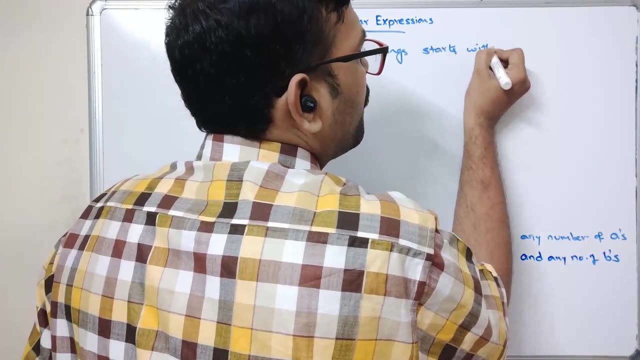 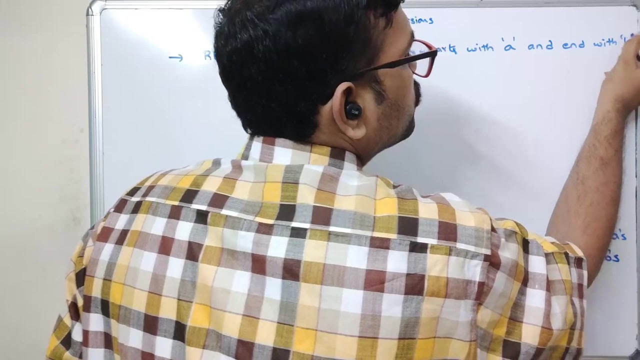 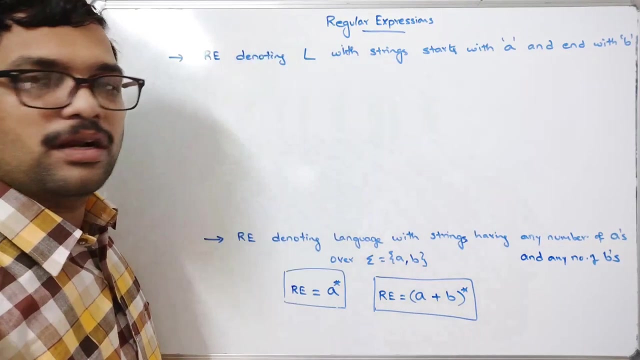 right. A language with a strings starts with A and end with B, so we need to write the regular expression. So previously we are supposed to construct the DFA or LFA for this particular question, so now we need to write the regular expression. see: 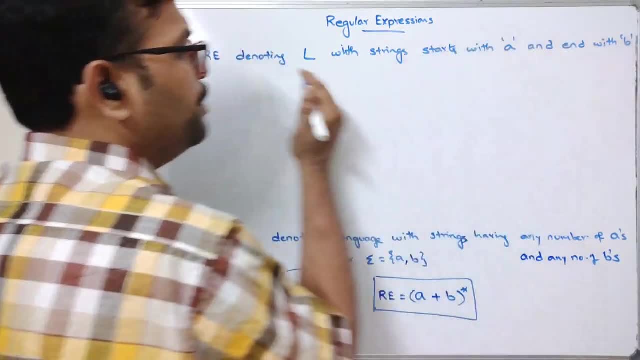 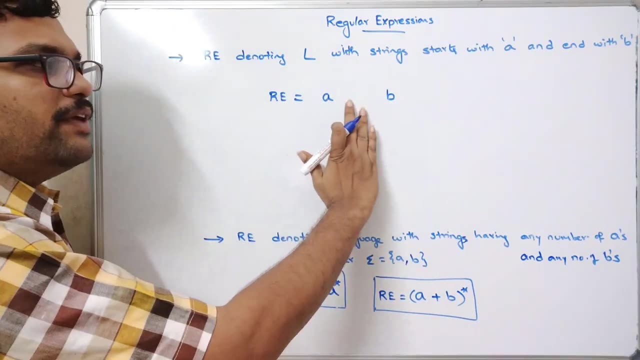 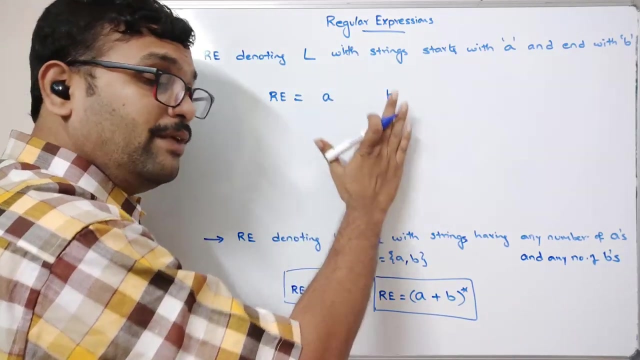 So here it is changed. It should start with A and end with B. so the regular expression will be: it should start with A, it should end with B, right, so in between there can be n number of A's and n number of B's, right? so it should start with A, it should end with B and in between it. 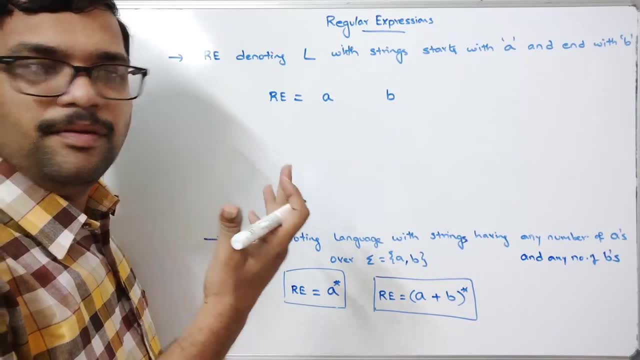 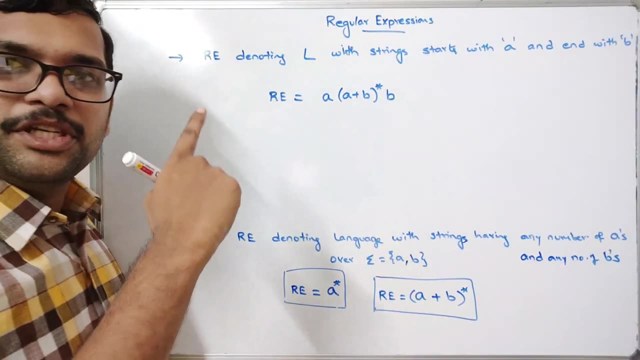 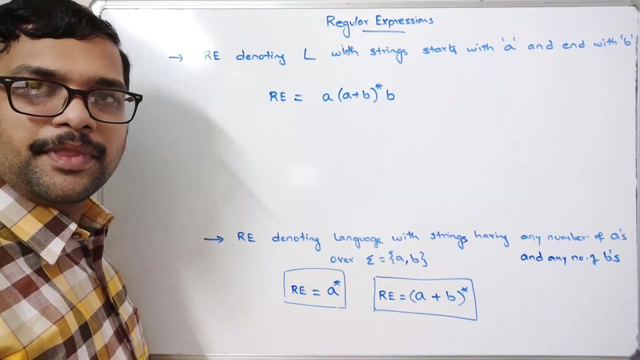 can be any number of A's and B's. the combination can be any, So simply we can write it as A plus B star. so this is the regular expression, which will have the strings which starts with A and ends with B. right, so this is a regular expression. 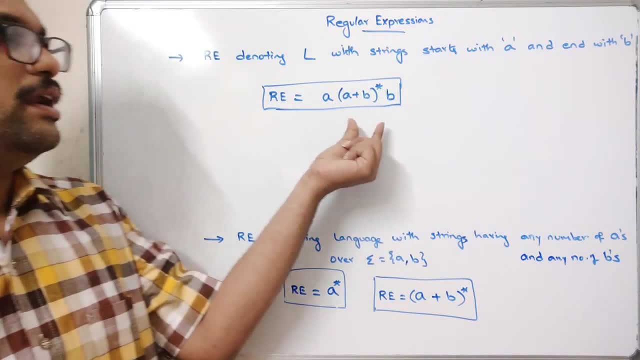 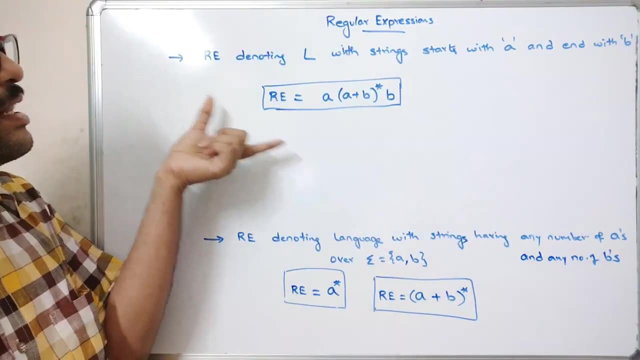 So we need to write the regular expression in the format right in this format. So previously we are writing the, we are constructing the DFA right. so now, in this case, the another thing, another way of representation, is the regular expressions. okay, set of characters. 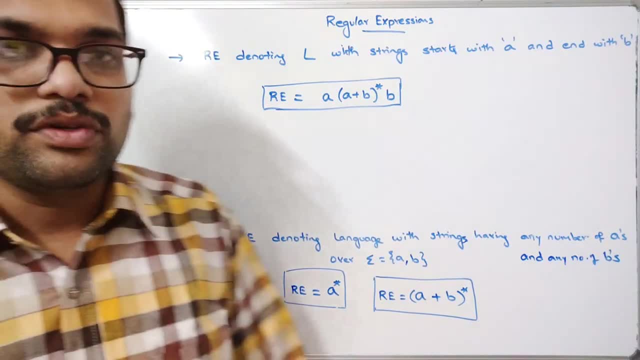 or a set of symbols, right, So now we have the regular expression. Okay, So hope you understood this one, and if you are having any doubt regarding this part, so feel free to post your doubts in the comment section. definitely, I will try to clarify. 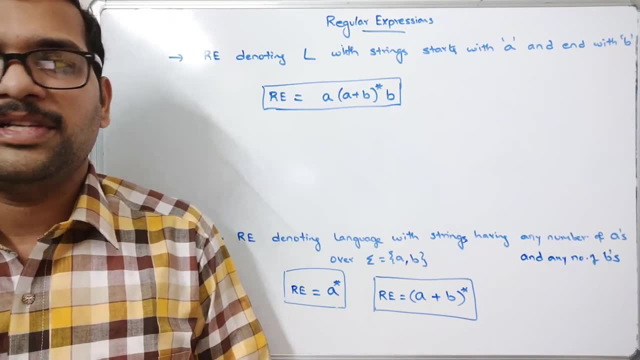 all your doubts And if you really enjoyed my session, like my session, share my session with your friends and don't forget to subscribe to our channel. Thanks for watching. Thank you very much. 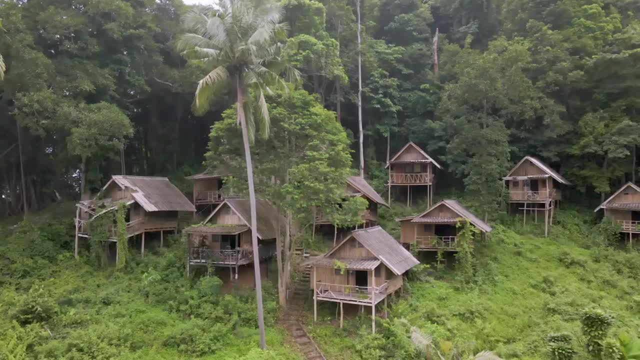 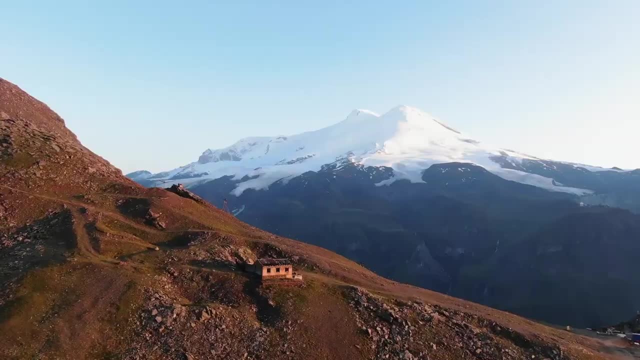 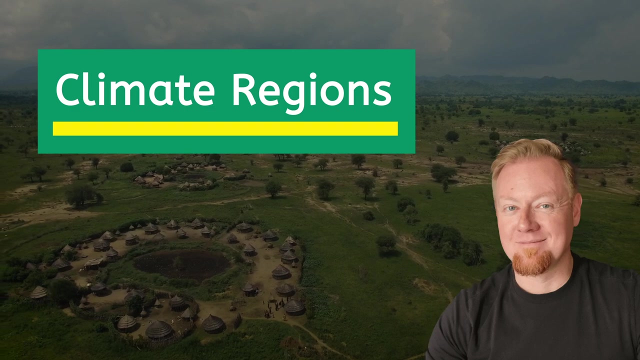 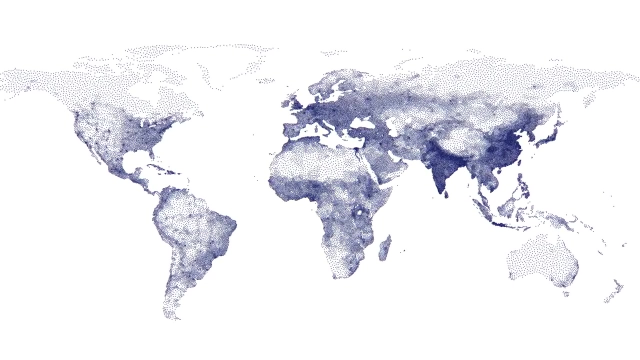 Hey there, explorers, It's Brian here with you for another adventure around the world. Look closely at this map of the world. You'll notice I've left off the title and a key. What information do you think this map displays? 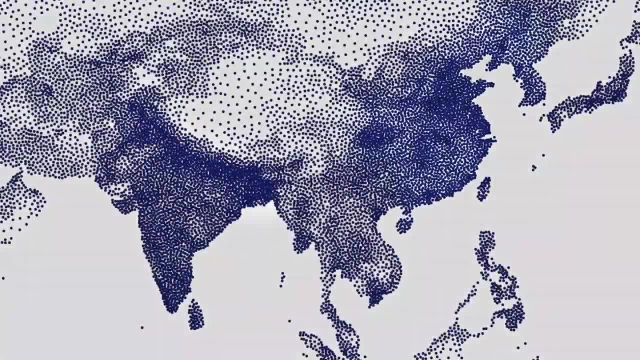 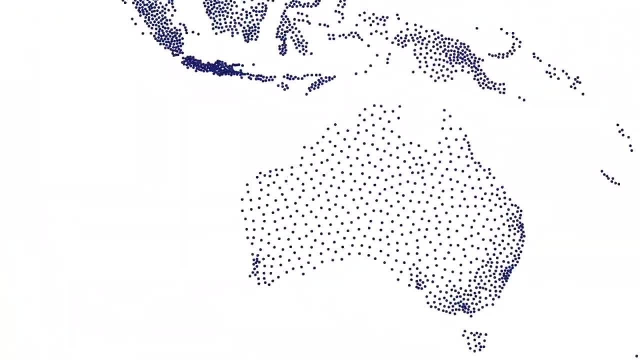 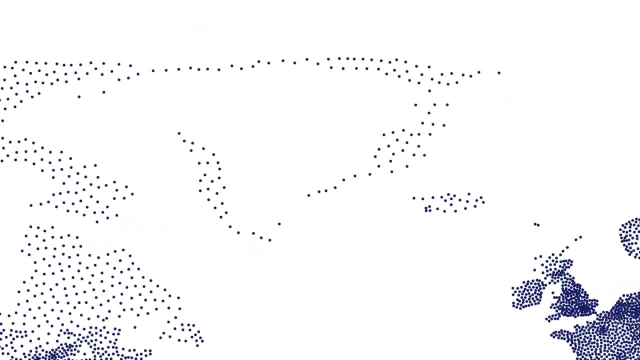 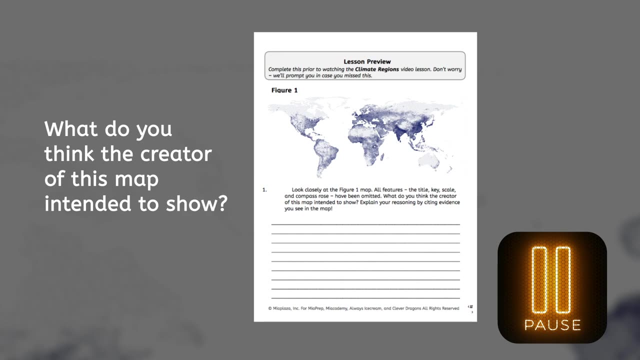 Go ahead, look for clues. You might notice that China and India have regions that are especially dark, and you might see that much of North Africa, Australia, Russia and Greenland are very light in color. If you haven't already completed the preview activity, pause the video here and write a. 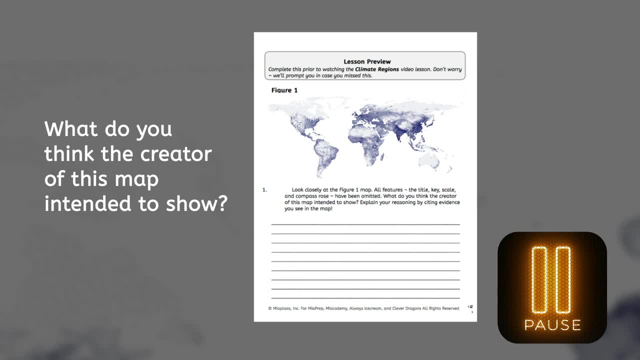 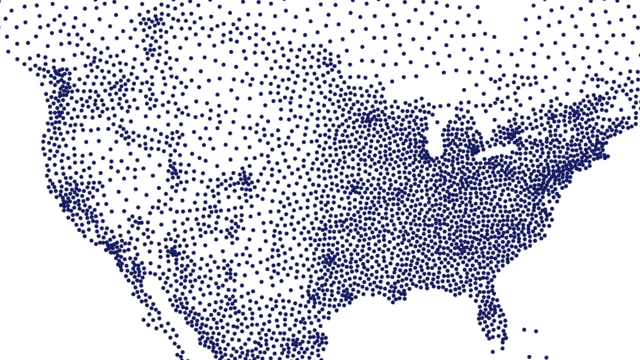 prediction about what you think this map is intended to show on the preview page of your PDF. Make sure to cite some evidence from the map to explain your reasoning. Let's zoom in on the US to see if we can figure this out. See the dark purple spots. 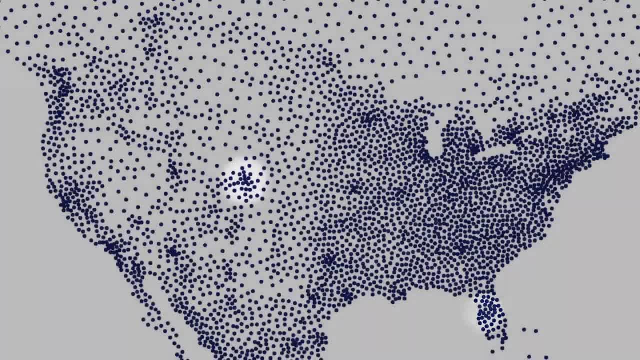 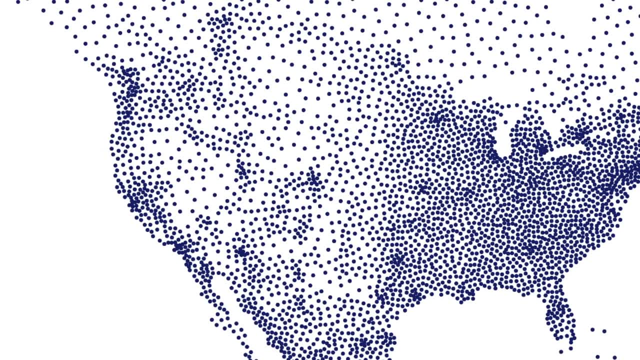 dotting the country. There's one here, another one here, and here There's a whole darkly shaded region up in the Northeast. Conversely, a lot of the West is pretty light in color, on the coast, where you can see much of California and some areas further north with dark coloration. 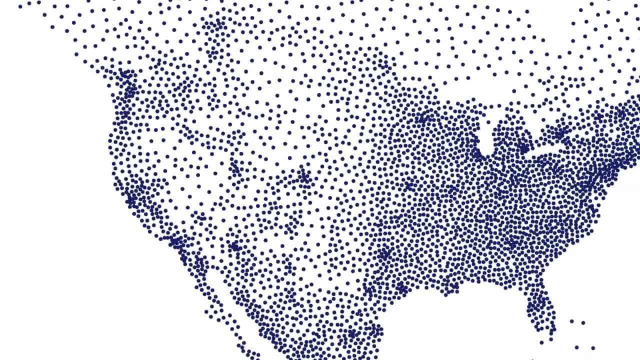 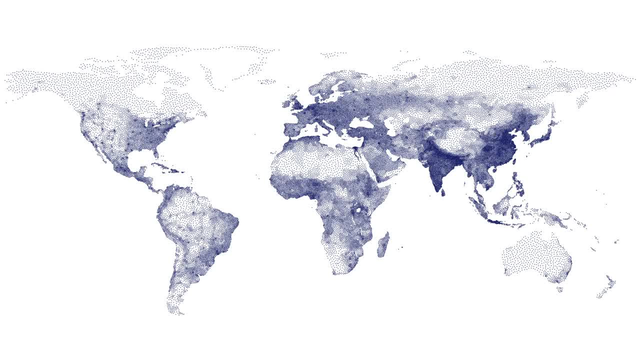 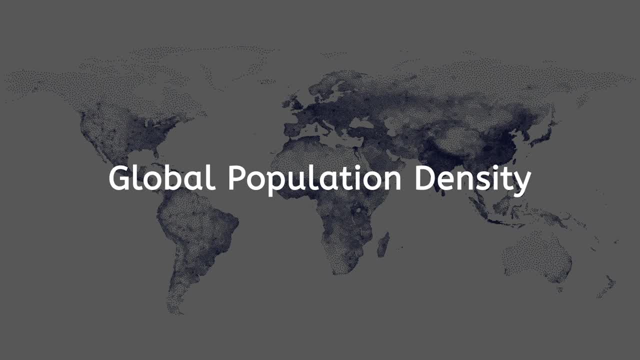 What do you think the dark areas represent? If you wrote in the preview that this map shows where people live, you're absolutely right. If this map had a title, it would be Global Population Density. The more people that live in a place, the darker the coloration appears on the map. You might even be able